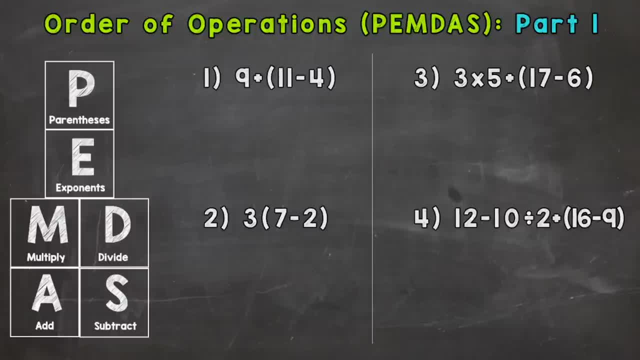 We have an acronym that helps us with these steps and it's at the top of your screen: PEMDAS, parentheses, exponents, multiply, divide, add and subtract. And there's also a graphic on the left side of your screen that will help us with these steps. 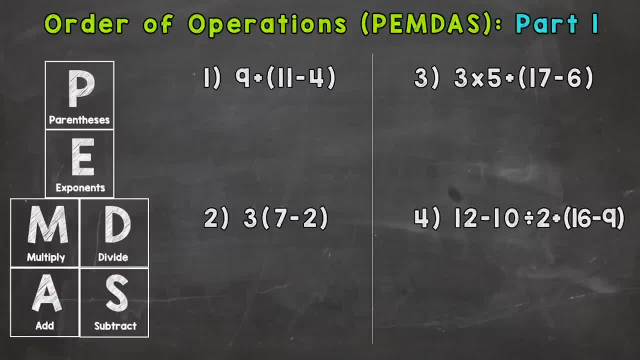 So parentheses is up top, That's number one priority. Whenever you see it in a problem, that comes first And then we work our way down that chart. Exponents is second priority. Level three is multiply and divide, And then we have add and subtract. So let's hop into number one. We have 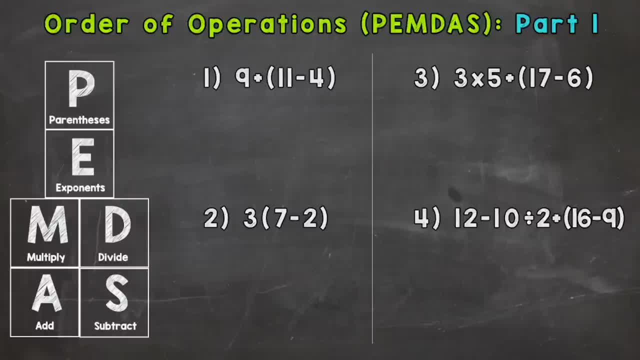 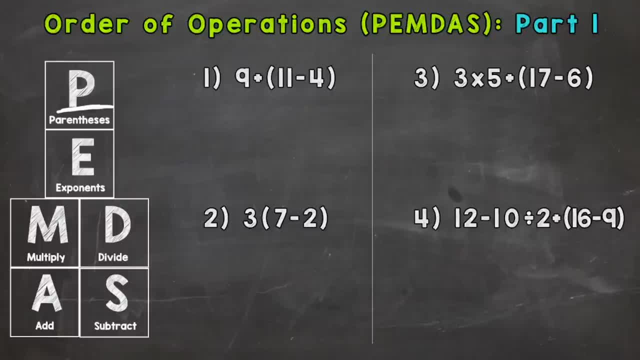 If you see parentheses in a math problem, that means it's number one priority. If you see parentheses in a math problem, that means it's number one priority. That's what you do first. So let's do eleven minus four first for number one. Eleven minus four is seven. 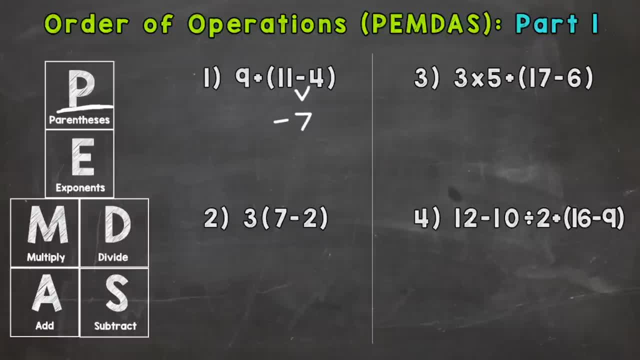 And now we need to bring down everything we did not use. So we did not use the plus, the addition, and we did not use the nine. Now we only have one operation left, So that's what we have to do. So let's end with nine plus seven, which is sixteen, And that is the answer to number one. 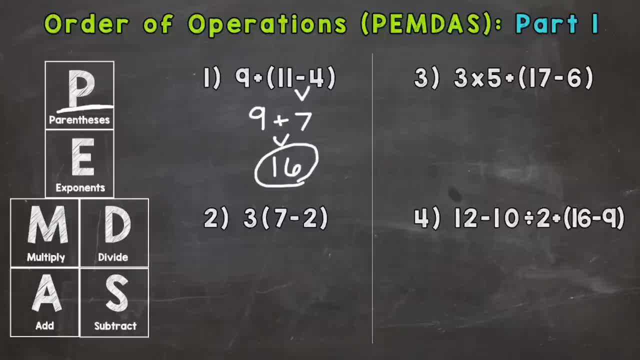 And that is the answer to number one. one number two: we have a three right next to a parenthesis and then seven minus two within those parentheses. so anytime you have a number right next to the parentheses that means multiply. so I'm going to rewrite the problem with a. 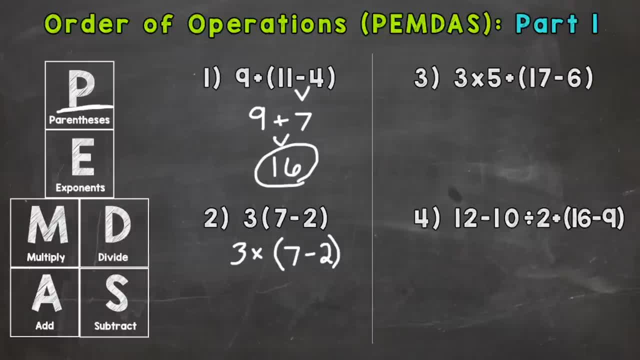 multiplication sign in there. so again, anytime you see a number right next to parentheses, it is multiplication. all right, so let's go through our steps. step one: parentheses: do we have any in this problem? yes, so that's what we need to do. first, seven minus two is five, and then let's bring down everything we 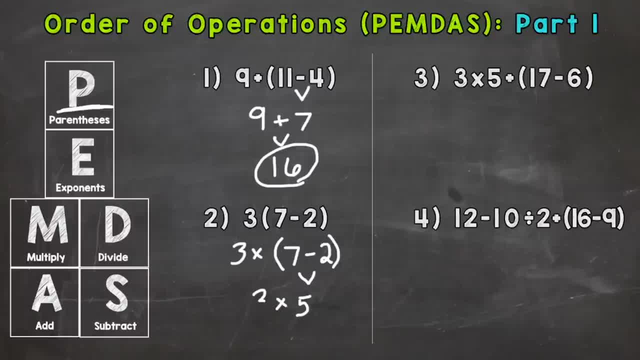 didn't use the multiply and the three, so we end with three times five, which is 15. so there you have it. there's number one and number two, so let's hop over to three and four. these get a little more complex and have more steps to them than numbers. 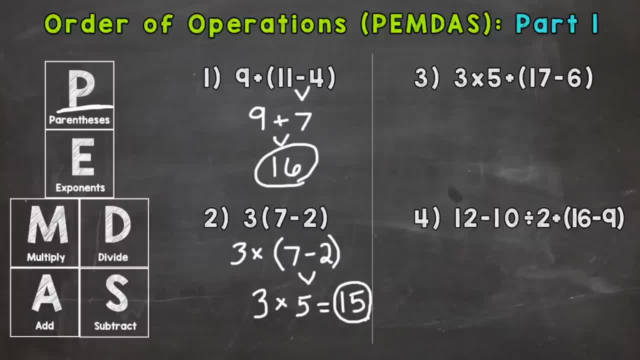 one and two. now it's important, with three and four and the more complex type of problems, to do one step at a time and make sure you're going through your process. so, number three: let's go through our steps, any parentheses. yes, so that's what we need to do. 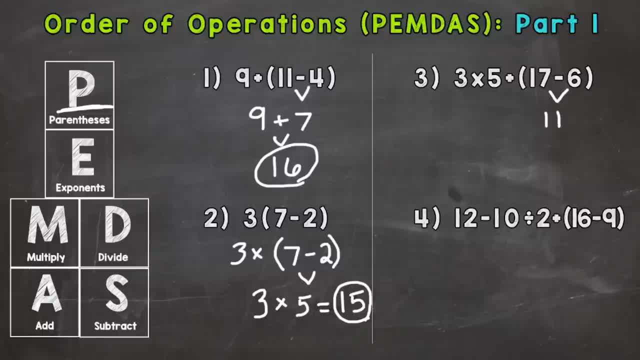 first: 15 minus six is 11.. let's bring down everything we did not use. so now we have multiplication and addition, so let's go through our steps. any parentheses now? no. any exponents: no, any multiplication or division. yes, so that's what we need to do. 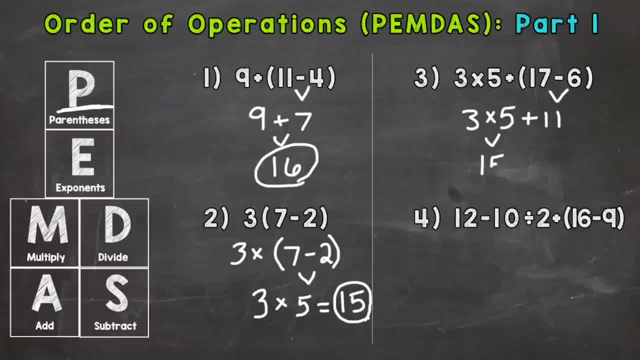 next. so three times five is 15.. drop whatever we haven't used yet, so we have 15 plus 11, which will get us to 26.. so number four: we have 12 minus 10, divided by 2 plus 16 minus 9 in parentheses. 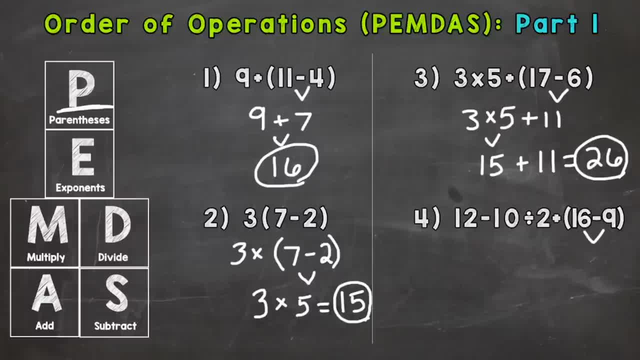 so parentheses we need to do first. 16 minus 9 is 7.. now we need to bring down everything that was not used, so let's try to reduce the number entre two and six. Once we're done, we're missing those engineers. does we have anything to say about these particular? 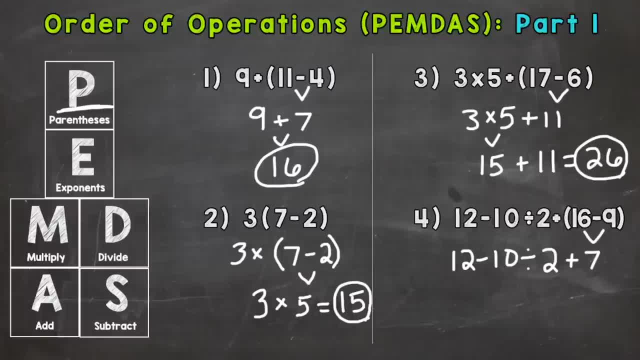 JA whабат. yeah, spl Abb 기다�. and so that plays into the power of division. so now we have subtraction division in addition. so any parentheses: no. any exponents, no, any multiplication or division. yes, so that's what comes next. 10 divided by two is 5. bring down everything we did not use. Everything Still needs to stay in the same order when rewriting the problem after you're going through your steps. so the 12 Boog, bla, bla is 10 divided by 2 is 5. bring down everything we did not use. Everything Still needs to stay. stay in the same order when you're rewriting the problem after you're going through our steps.